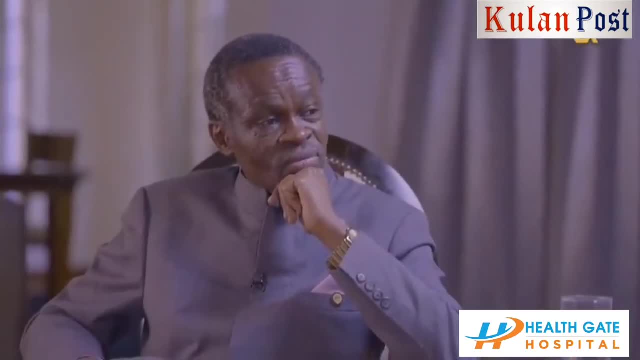 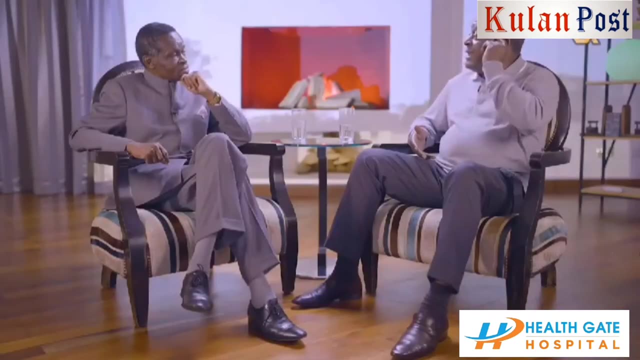 And he made noise All through. I just thought he's being unreasonable, Giving him documents. he needs to find out. But then, when I was leaving, is when my head opened up because I was told: whatever we have discussed here, if I hear it out there, you will know. 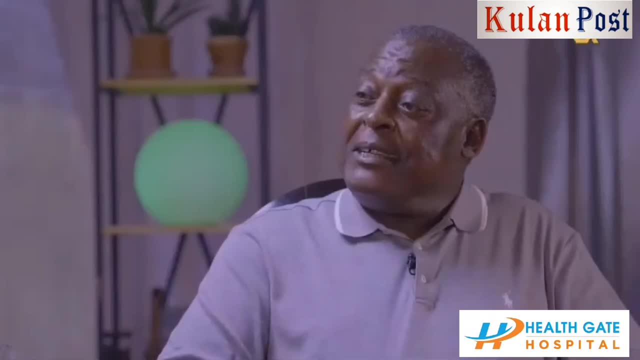 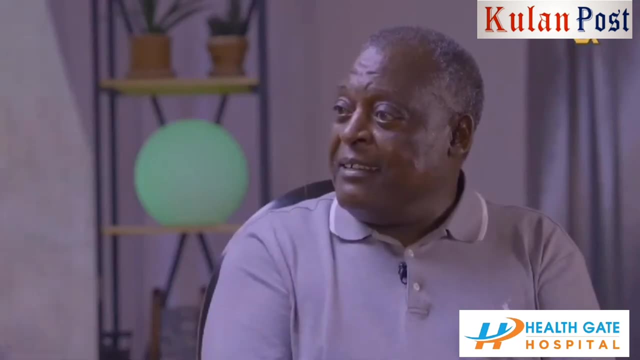 So I left. Then I said: what was I doing? Did I go to talk to whoever was dumping the toxic waste that we are dumping toxic waste here? Because that appeared to be the reason, Because the way the whole information was received was so violent. 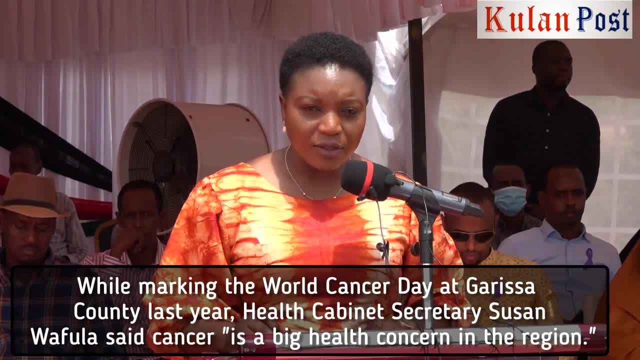 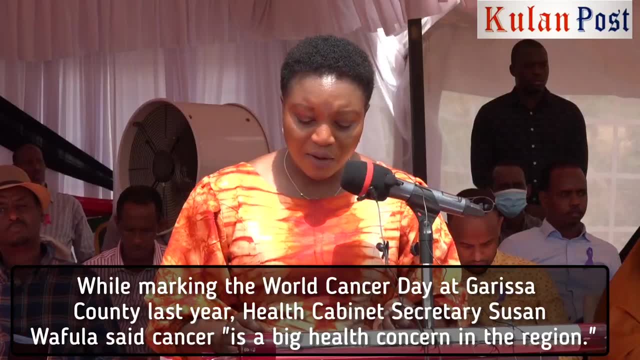 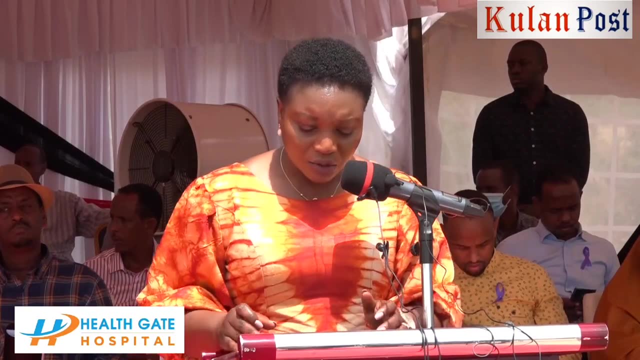 These results are the leading causes of illness and death. globally, These results in estimated 41 million. The burden of cancer is rising over the past few decades And it's projected to get even higher, as we were told by our chief, the executive director of this hospital. 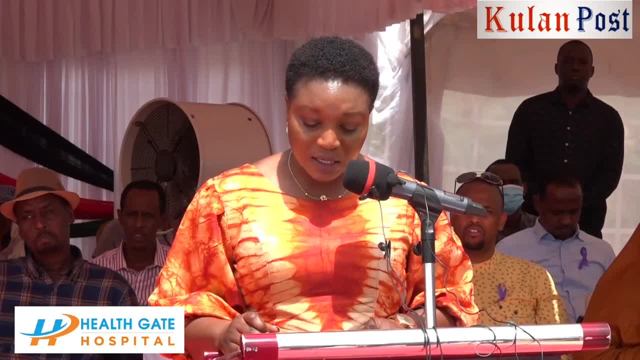 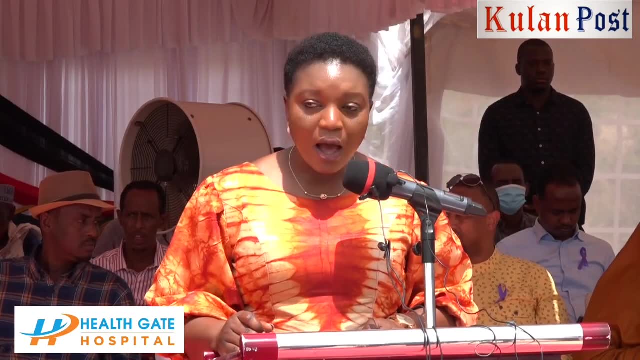 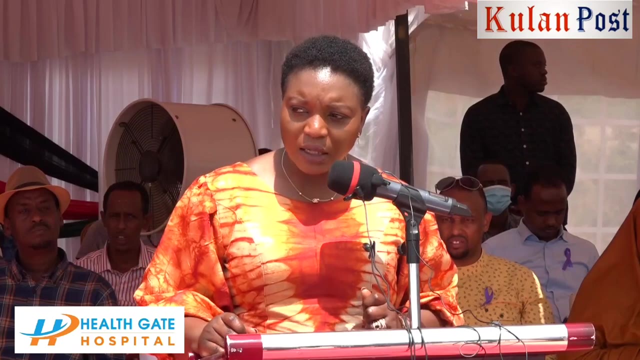 Here in Garissa we mostly see cancers of the head and neck And I am concerned that they presenting very late to our facilities. I know that we can change this experience And I listened to the CEC for health on what he did in creating awareness in the local language. 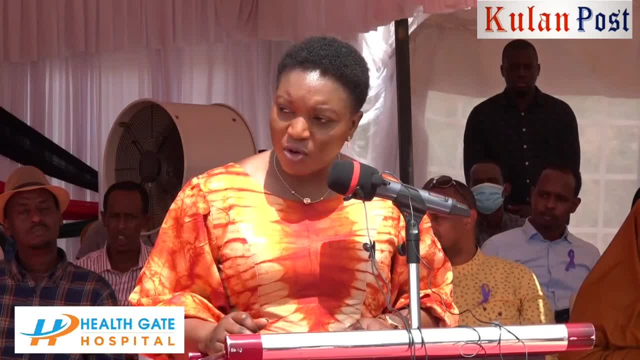 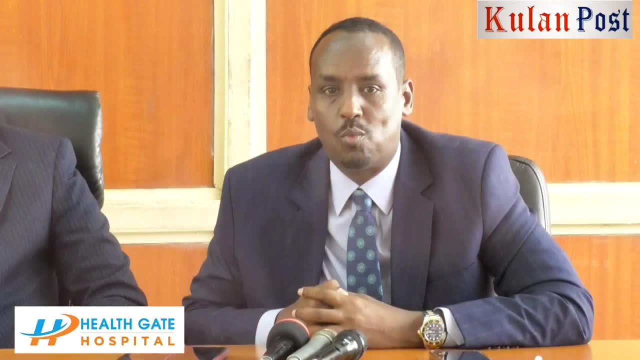 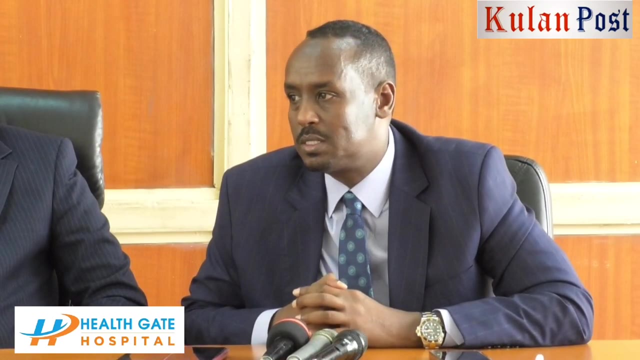 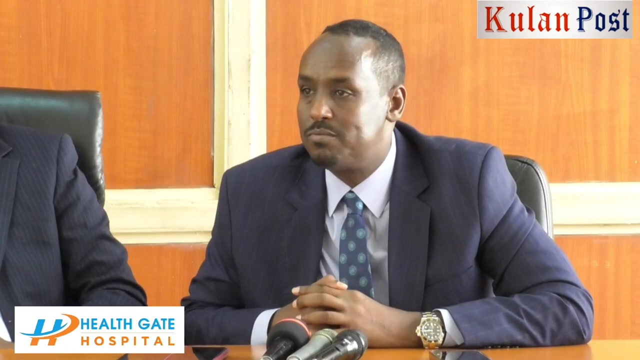 I've also listened to the member of parliament and I want to congratulate them and say: let us continue creating our awareness so that our people can get treatment. What Jurongo alleged in that interview, that recent interview, is something that has been going. I mean, it's part of the rumor mills, if I can say. 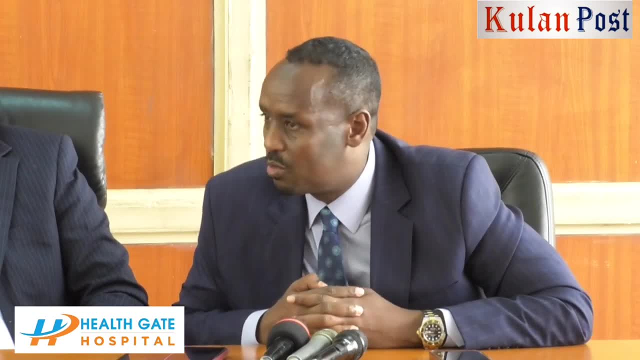 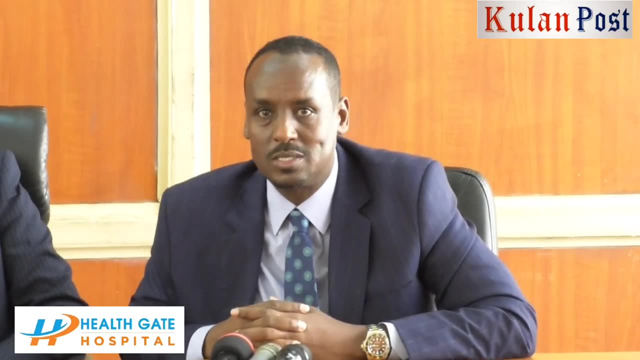 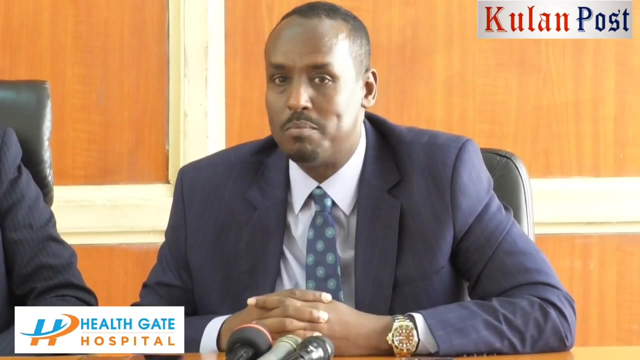 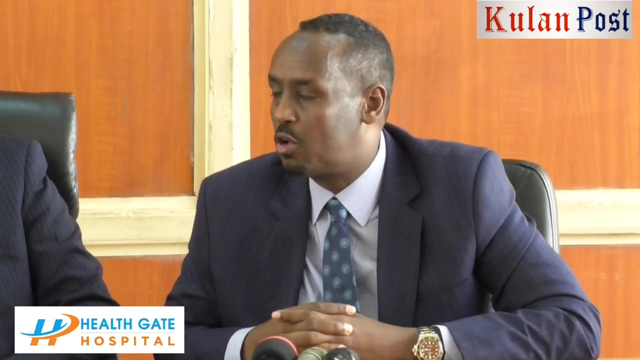 And the claims and counterclaims we've kept hearing as we grew up in northeastern Kenya over the years about the existence of nuclear or toxic waste buried in the midst of our region. Places that we've had before include parts of Garissa, particularly the northern part of Garissa.